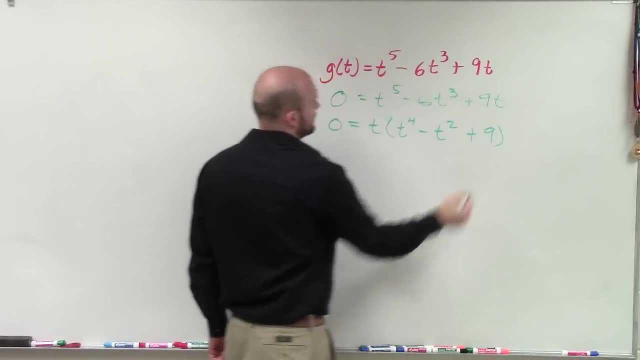 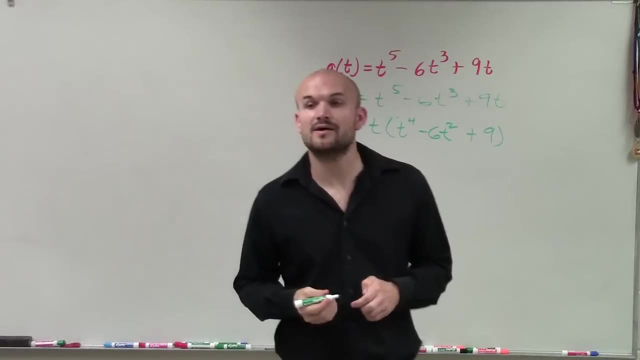 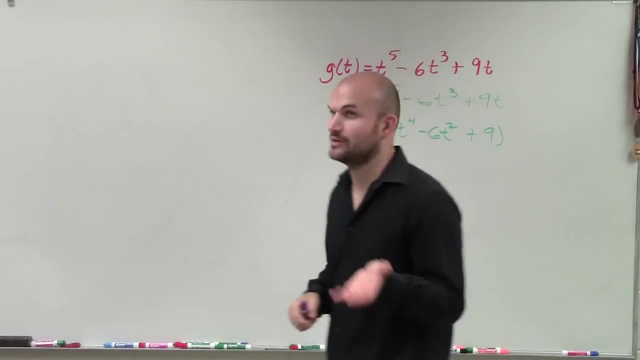 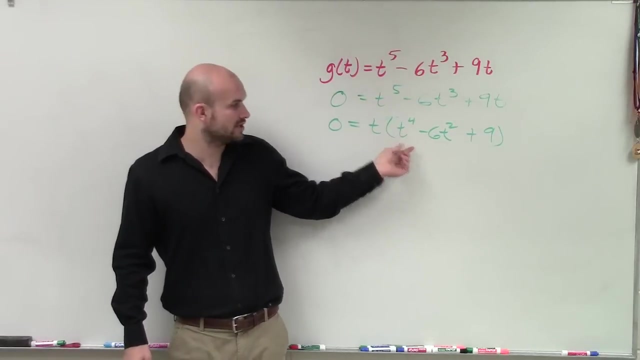 So I have t to the fourth minus t, squared plus nine. Now, I'm sorry, that's a 60, right, 60 squared, All right. so now I need to factor this. Well, I gave you that worksheet, Remember, on perfect square trinomials: A squared minus two times, or a squared plus or minus two, two a, b plus b squared. Well, notice that John T to the fourth is a squared term, Nine is a squared term And the negative six, t squared. 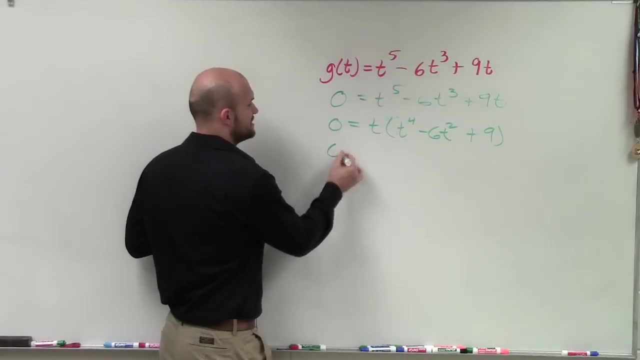 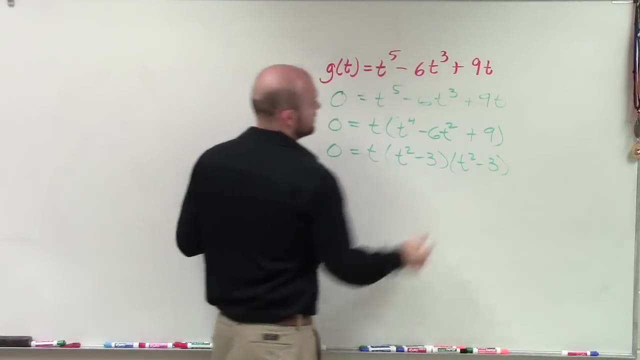 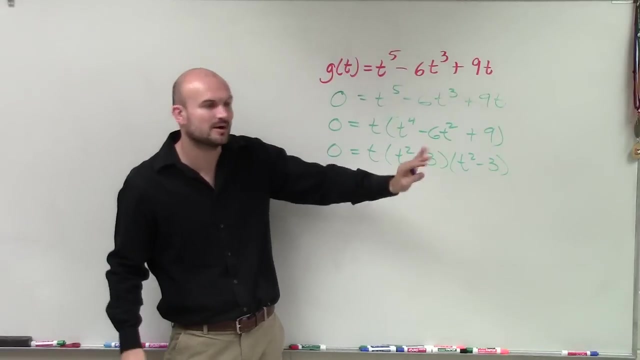 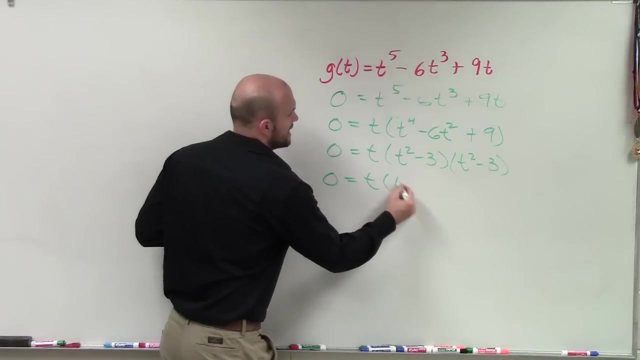 is two times a times t or a times b. So therefore I can factor this as: zero equals t times t squared minus three times t squared minus three. Now again, yes, that's the factored form. You guys can do the x if you want to do the x, And you can convert this to t squared if you want to. But now we have t squared minus, or sorry, t squared minus, three times t squared minus three. So we have zero equals t times t squared minus three squared Right, All right. so 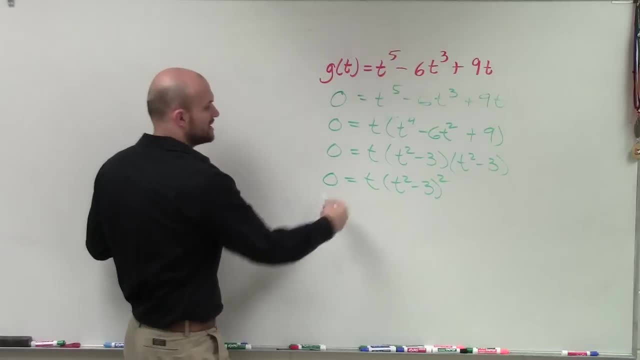 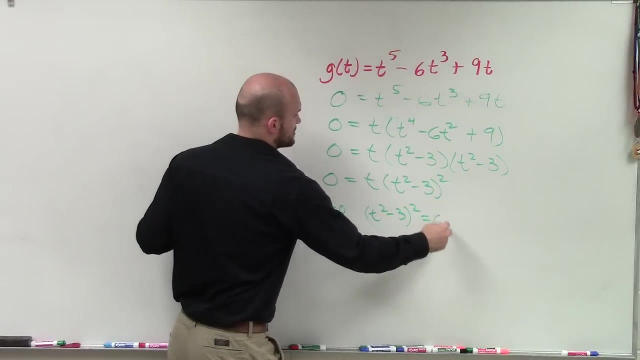 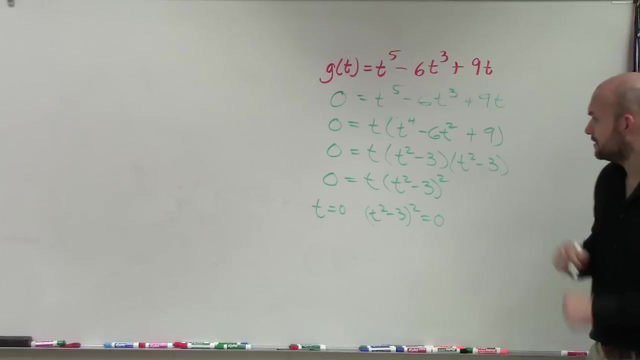 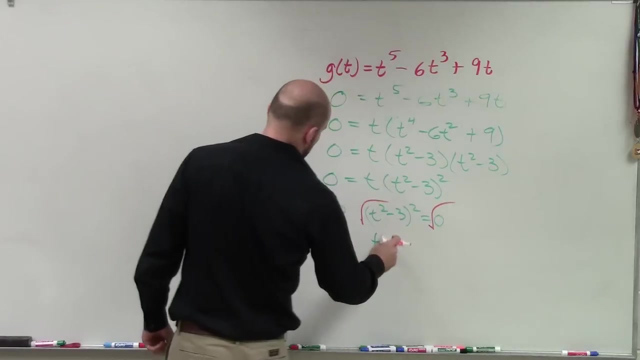 we are going to determine. let's go ahead and first find the zero. So I apply zero product property: t equals zero, And t squared minus three squared equals zero. So now in this case I solve. I already solved t equals zero. So that's easy. Here I'm going to have to apply my inverse operations, So I'll take the square root of both sides. Then I'm left with t squared minus three equals squared. zero is just zero. Then I add three. 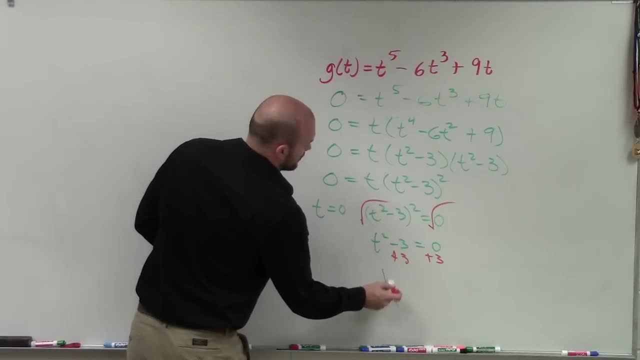 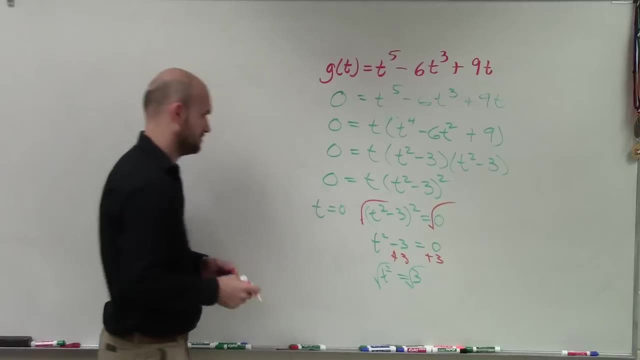 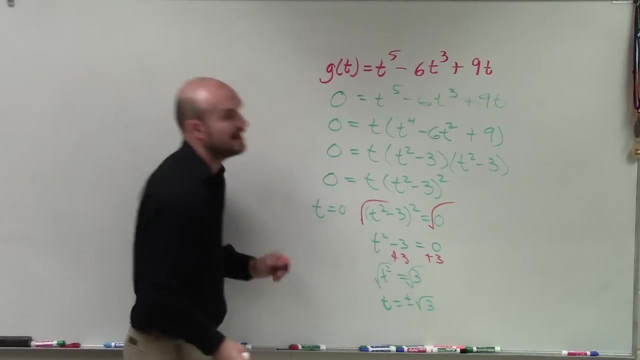 t squared equals a positive three. Take the square root. Take the square root. t equals plus or minus the square root of three. Now, those are two different zeros. right, Let's look again at the multiplicity of their factor. The multiplicity of their factor is a what Two. So you could say that these two- I'm not going to write multiplicity- 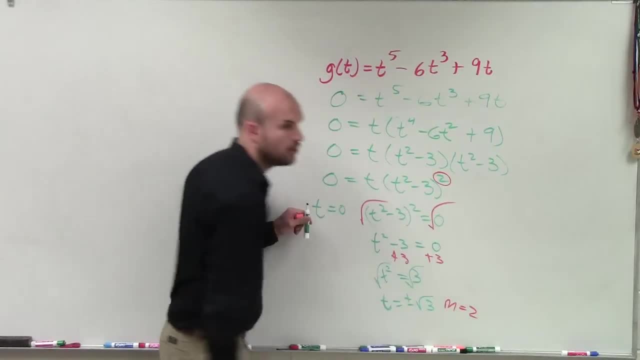 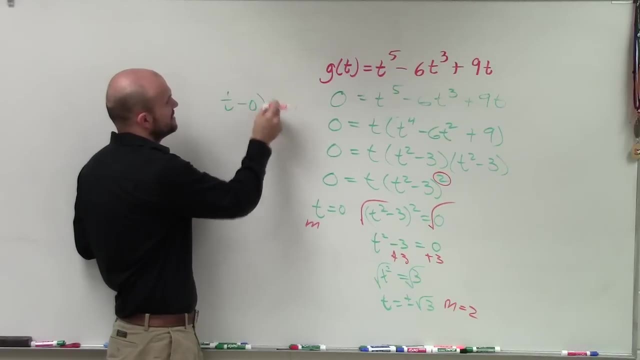 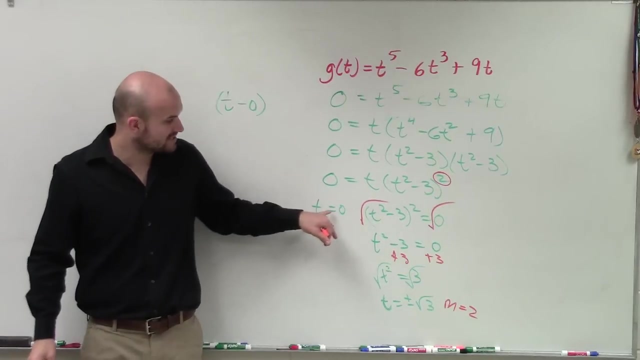 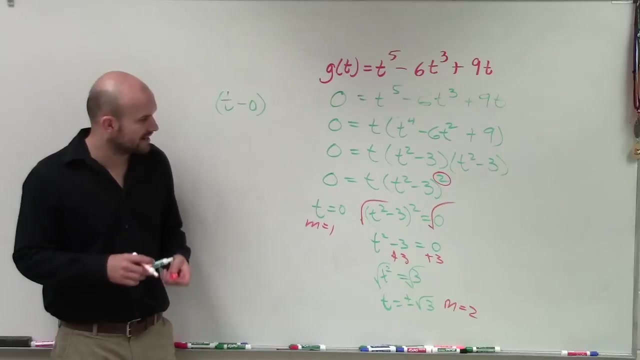 I'll say m. The multiplicity of here is two, Or even here we have a multiplicity that was one, Right? Because, remember, t can be written as t minus zero, Right? So therefore this multiplicity is equal to one. So therefore the graph crosses at t equals zero and then touches at plus or minus the square root of three.